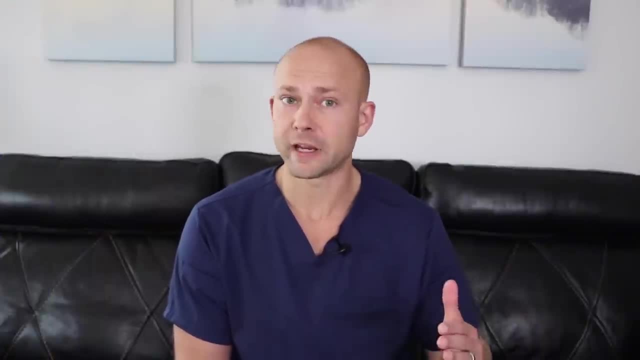 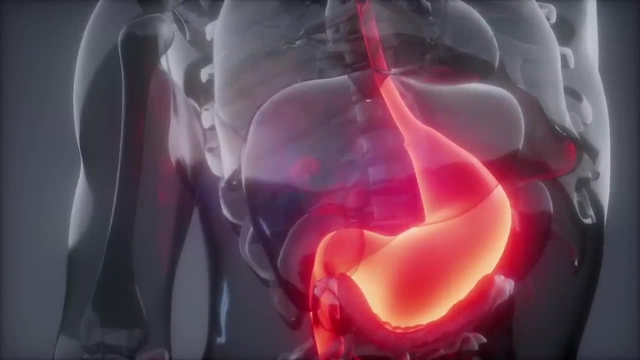 I knew right away there was a problem, A problem that would prevent her from drinking apple cider vinegar until some healing was done. What was occurring is an ulcer. An ulcer is a sore that develops in the stomach, in the esophageal lining or maybe even in the 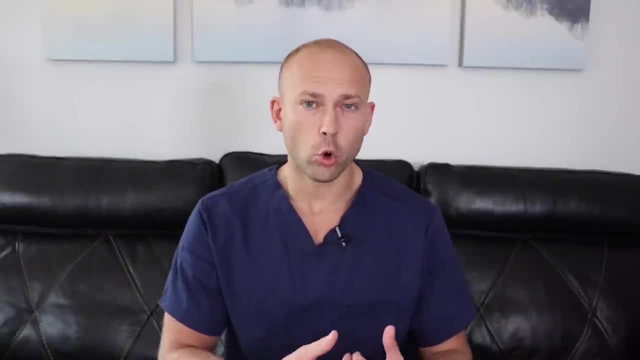 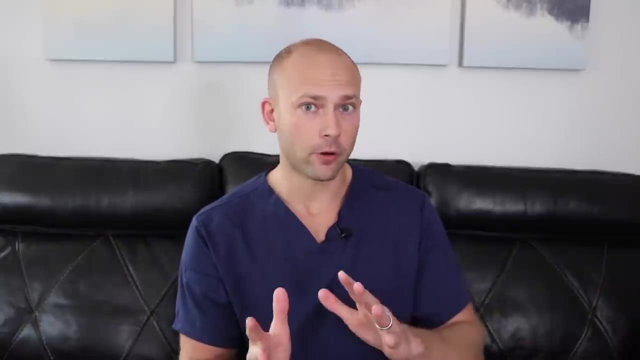 small intestine And when you drink something like apple cider vinegar or anything acidic, maybe even a kombucha- what happens is you get an intense burning feeling. So you have to back off from apple cider vinegar or anything acidic until some healing is done And of 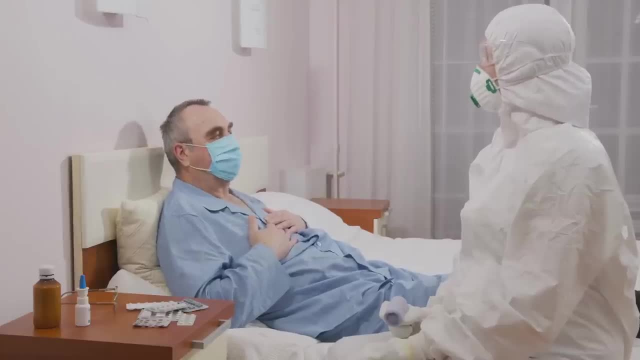 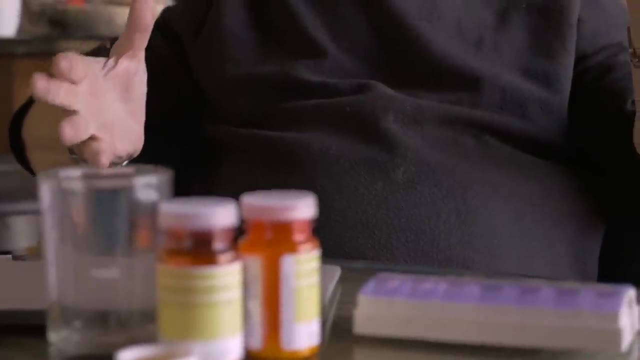 course, we're talking about the health of your stomach, your liver, your whole body, your natural healing. Now, due to the chronic illness plague that we face as a society, the average person is on four or more prescription medications. What we have to really be careful with here is 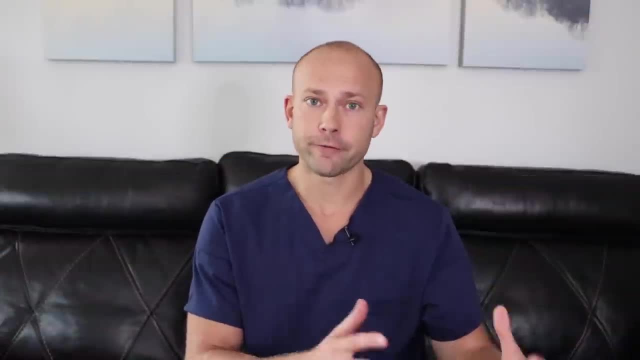 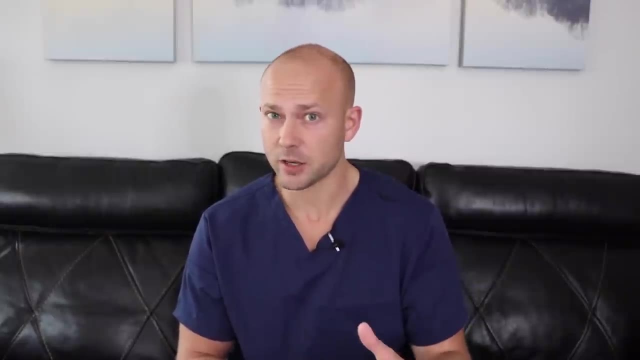 interactions. If you're recommending apple cider vinegar to a friend or a family member, then you may want to realize that there could be some potential complications at stake here. An example of this might be somebody who's a diabetic- a type 2 diabetic- who's taking insulin. 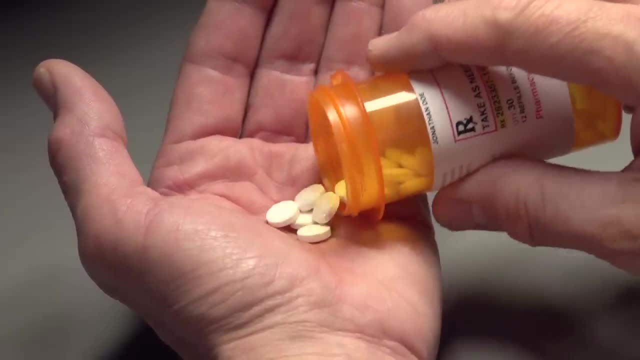 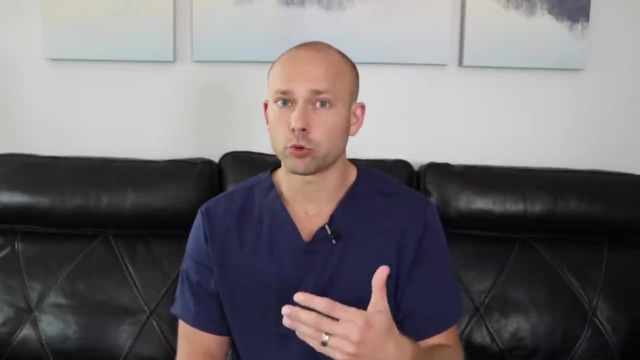 or maybe taking some sort of drug to drive down their blood sugar. If you combine that with apple cider vinegar, you could drop your blood sugar to a very low and unhealthy place. Maybe you're taking a drug to lower potassium levels and then combining that with apple cider vinegar could. 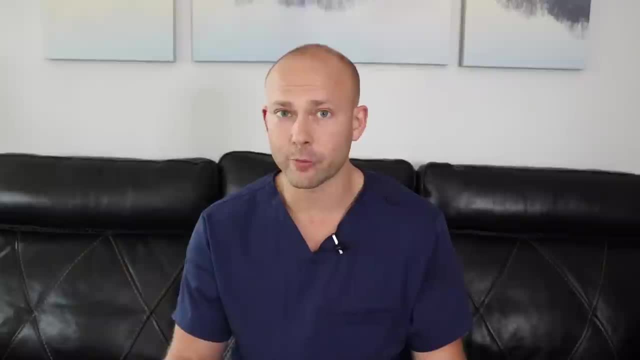 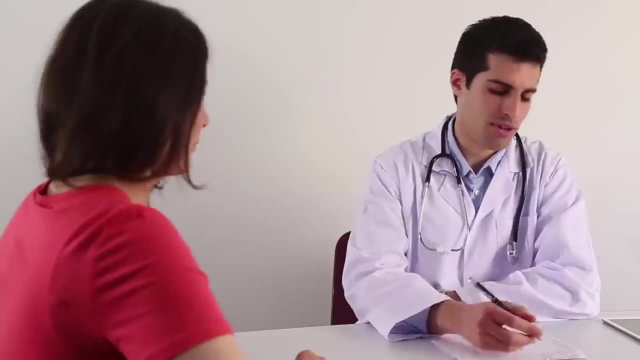 drive the potassium levels too low. The same goes with like a diuretic, So we just have to be careful and always ask your doctor if you have any questions regarding a medication and how it actually interacts with a particular food or beverage that you want to drink. 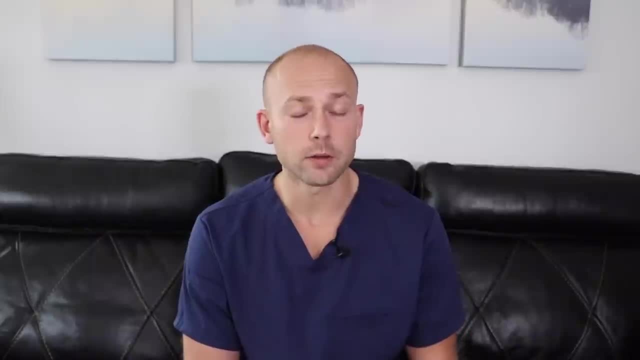 So there were this girl. she's 15 years old and she wanted to lose some weight, So in order to do so, she started drinking one cup- Now you're hearing this right- one cup of undiluted apple cider vinegar every single day. As a result of that, she had severe tooth decay. Another scenario is a 28. 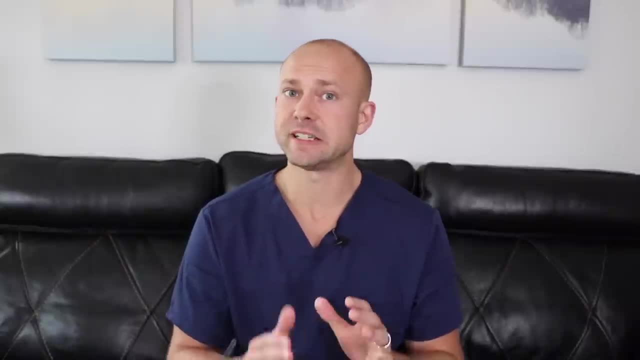 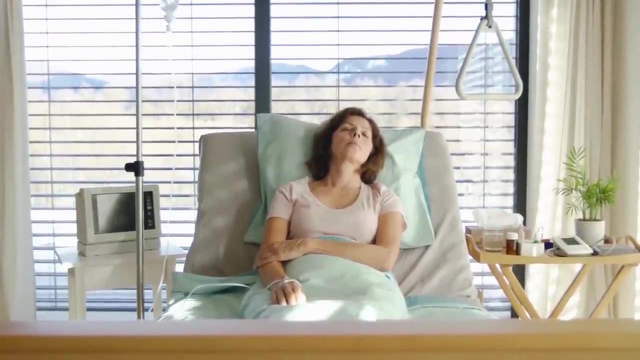 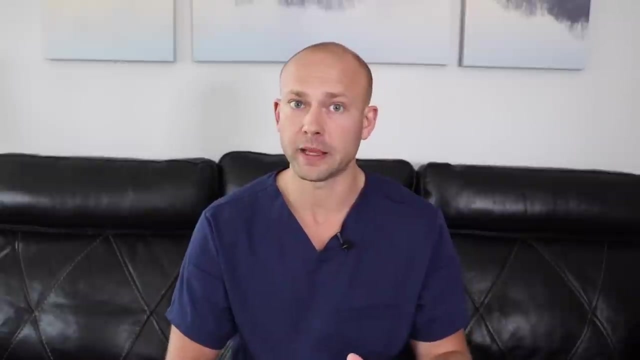 year old woman who had drank eight ounces of apple cider vinegar daily for six years straight. She was admitted to the hospital for having low potassium levels. Now, upon further analysis, what they found in the hospital is that she actually had brittle bones and it was believed to be due to over consuming apple cider vinegar.